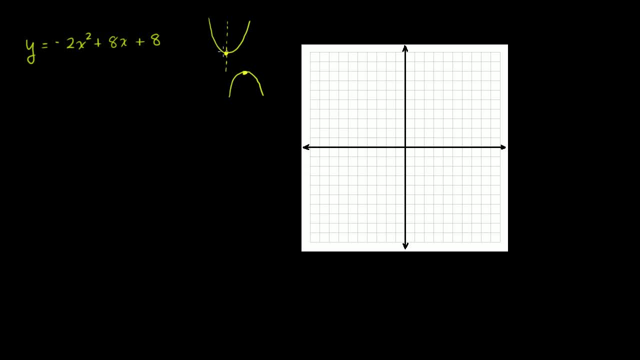 So that's the axis of symmetry, That is a reflection of the left-hand side along that axis of symmetry. Same thing if it's a downward opening parabola. And the general way of telling the difference between an upward opening and a downward opening parabola is that this will have a positive. 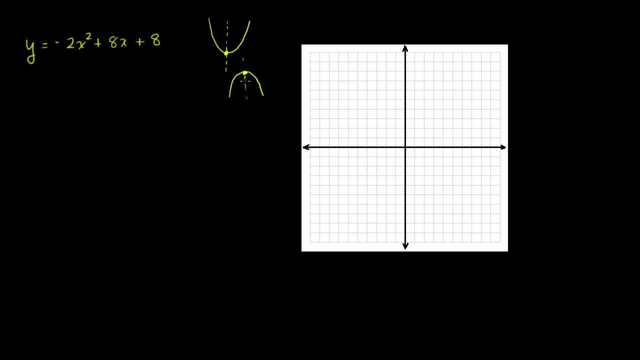 coefficient on the x squared term and this will have a negative coefficient, And we'll see that in a little bit more detail. So let's just work on this Now In order to figure out the vertex. there's kind of a quick and dirty formula. 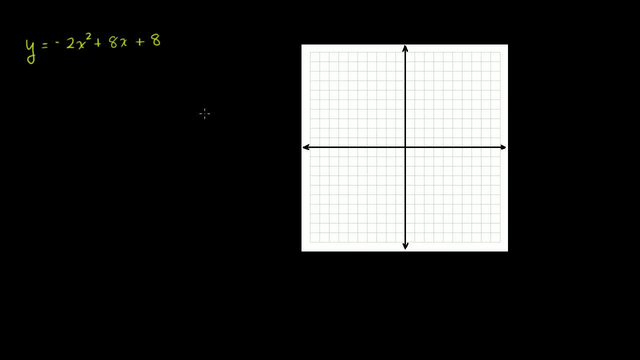 But I'm not going to do the formula here, because the formula really tells you nothing about how you got it. But I'll show you how to apply the formula at the end of this video, if you see this on a math test and just want to do it really quickly. 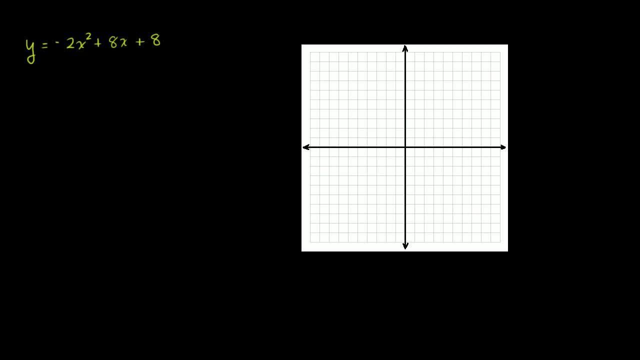 But we're going to do it the slow and intuitive way first. So let's think about how we can find either the maximum or the minimum point of this parabola. So the best way I can think of doing it is to complete the square. 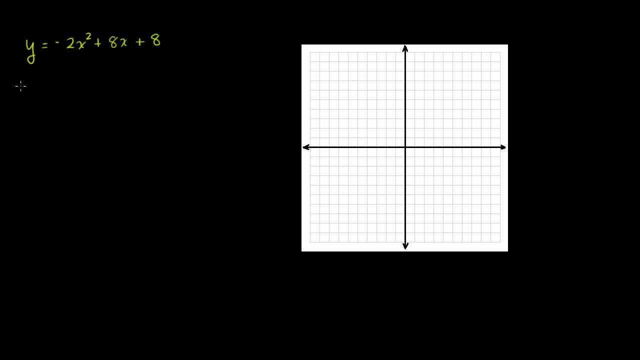 And it might seem like a very foreign concept right now, But let's just do it one step at a time, So I can rewrite this as y is equal to well, I could factor out a negative 2.. It's equal to negative 2 times x squared minus 4x minus 4.. 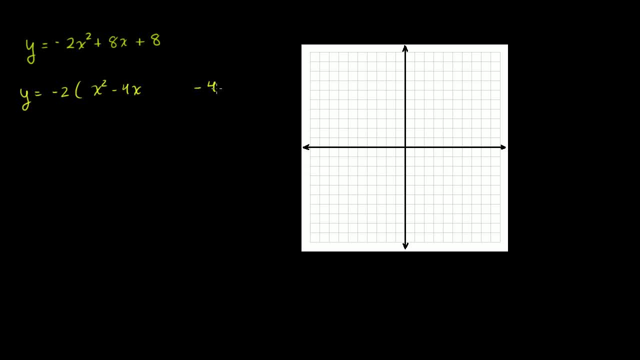 And I'm going to put the minus 4 out here, And this is where I'm going to complete the square. Now what I want to do is express this stuff in the parentheses as a sum of a perfect square, and then some number over here. 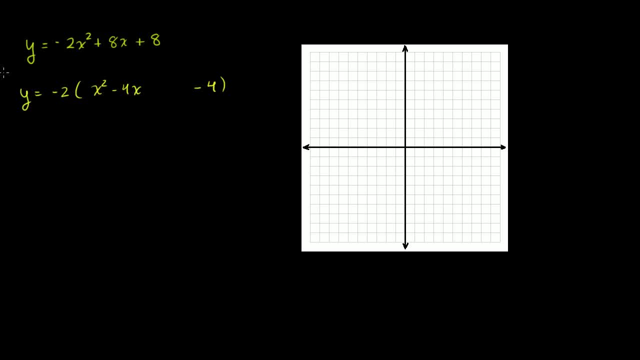 And I have x squared minus 4x. If I wanted this to be a perfect square. If I wanted this to be a perfect square, it would be a perfect square if I had a positive 4 over here. If I had a positive 4 over there, then this would be a perfect square. 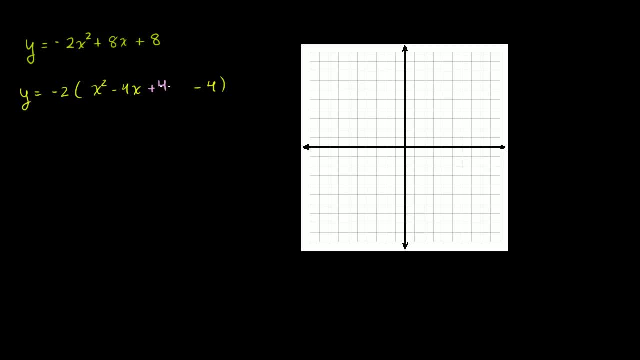 It would be x minus 2 squared And I got the 4 because I said: well, I want whatever half of this number is. So half of negative 4 is negative 2.. Let me square it, That'll give me a positive 4 right there. 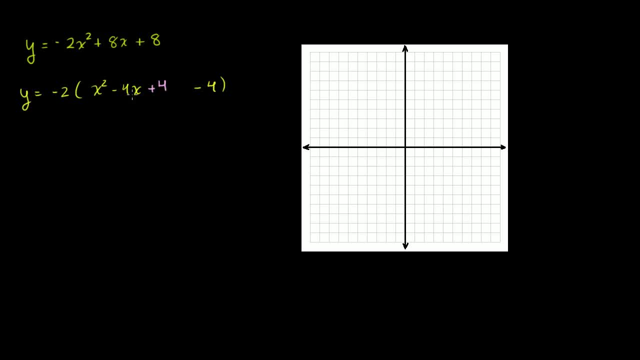 But I can't just add a 4 willy-nilly to one side of an equation. I either have to add it to the other side or I would have to then just subtract it. So here I haven't changed the equation, I added 4.. 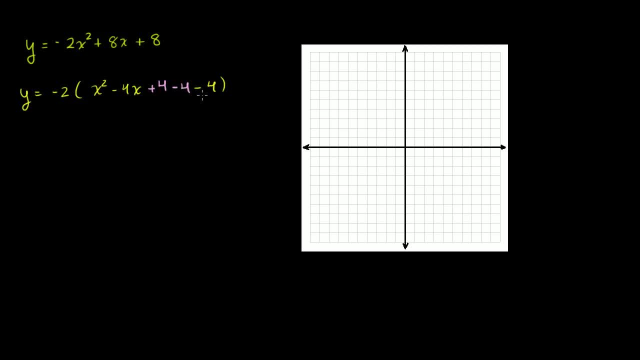 I just subtracted 4.. I just added 0 to this little expression here, So it didn't change it, But what it does allow me to do is express this part right here as a perfect square: x squared minus 4x plus 4 is x minus 2 squared. 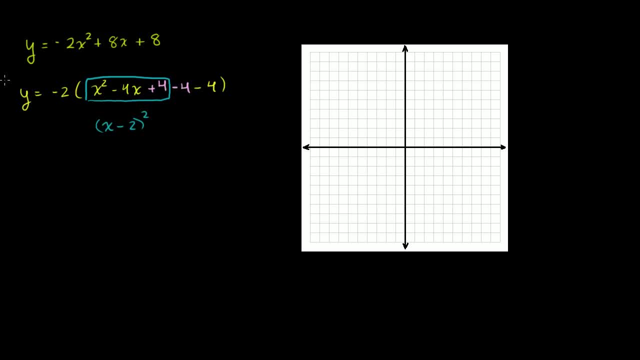 It is x minus 2 squared, And then you have this negative 2 out front multiplying everything, And then you have a negative 4 minus negative 4. Minus 8.. Just like that. So you have: y is equal to negative 2 times this entire thing. 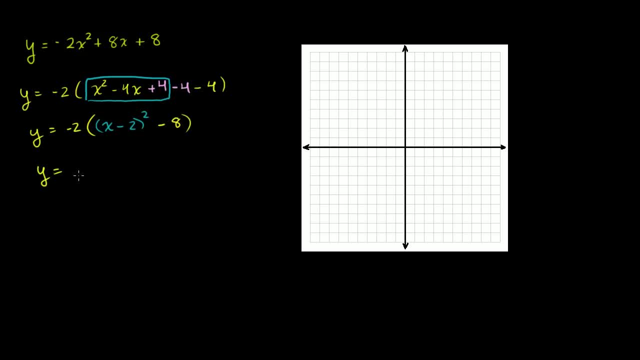 And now we can multiply out the negative 2 again, So we can say, we can distribute it: y is equal to negative 2 times x minus 2 squared, And the negative 2 times negative 8 is plus 16.. Now all I did is algebraically rearrange this equation. 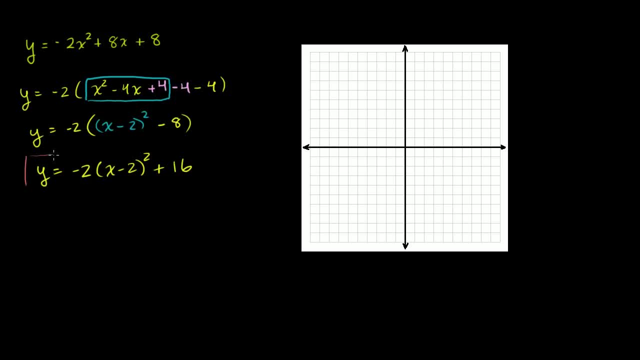 But what this allows us to do is think about what the maximum or minimum point of this equation is. So let's just look at- let's explore this a little bit- This quantity right here: x minus 2 squared- If you're squaring anything, this is always going to be a positive quantity. 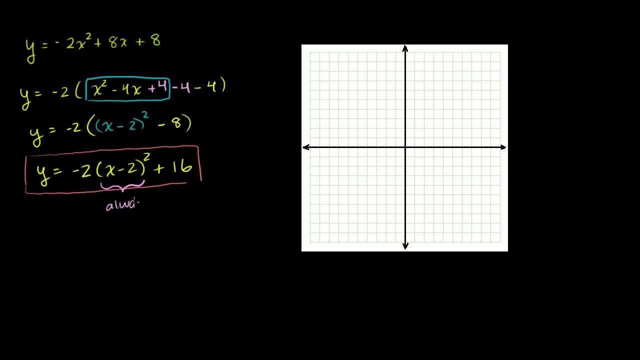 That right, there is always always positive, But it's being multiplied by a negative number. So if you look at the larger context, if you look at the always positive multiplied by the negative 2, that's going to be always, that's going to be always negative. 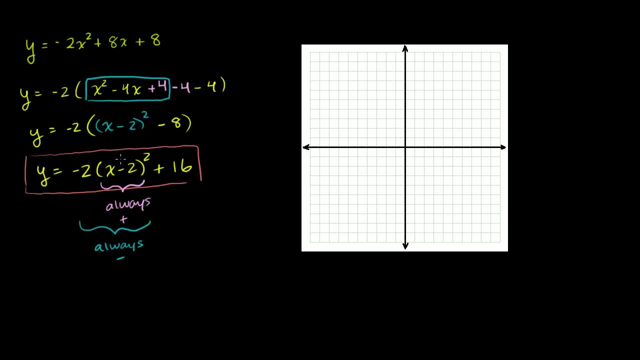 And the more positive that this number is, the more positive this number becomes When you multiply it by negative, the more negative this entire expression becomes, The more negative this entire expression becomes. So, if you think about it, this is going to be a downward opening parabola. 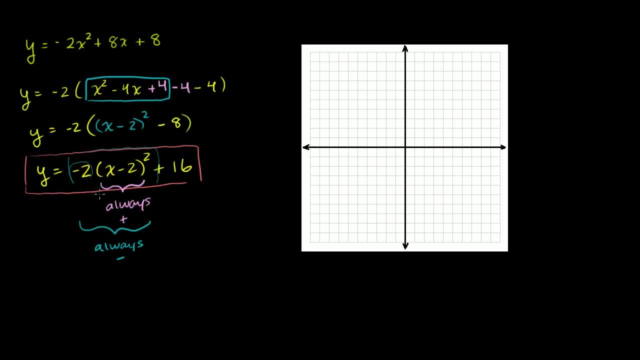 We have a negative coefficient out here, And the maximum point on this downward opening parabola is: when is when this expression right here is as small as possible. If this gets any larger, it gets multiplied by a negative number and then you subtract it from 16.. 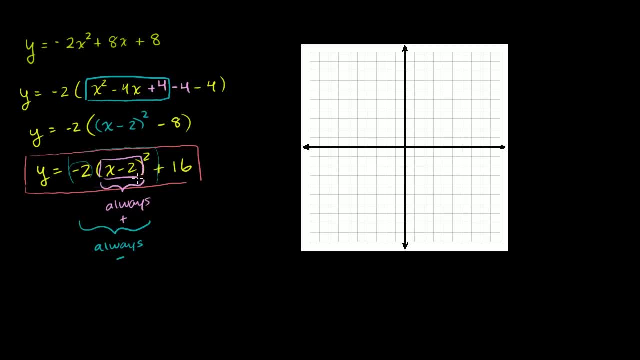 So if this expression right here is 0, then we have our maximum y value, which is 16.. So how do we get x is equal to 0 here? Well, the way to get x minus 2 equal to 0, so let's just do it. 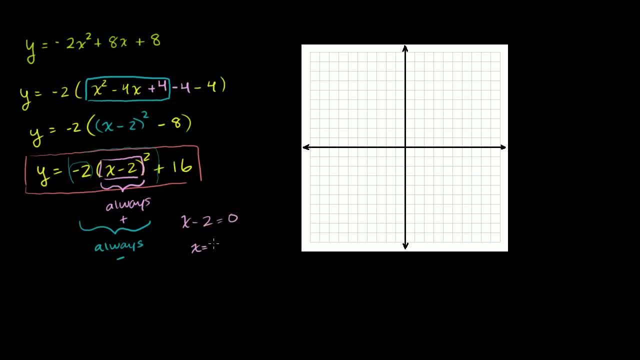 x minus 2 is equal to 0, so that happens when x is equal to 2.. So when x is equal to 2, this expression is 0,, 0 times a negative number, it's all 0, and then y is equal to 16.. 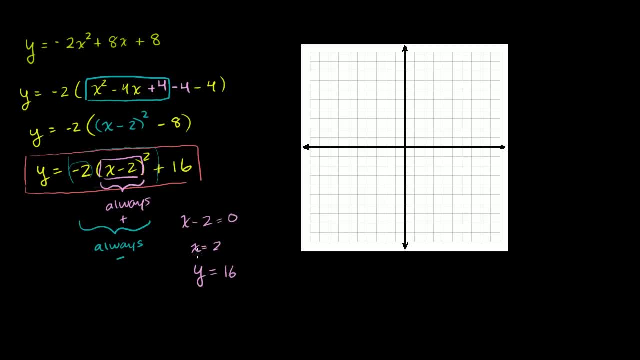 y is equal to 16.. This is our vertex. This is our maximum point. We just reasoned through it, just looking at the algebra, that the highest value this can take on is 16.. As x moves away from 2 in the positive or negative direction, 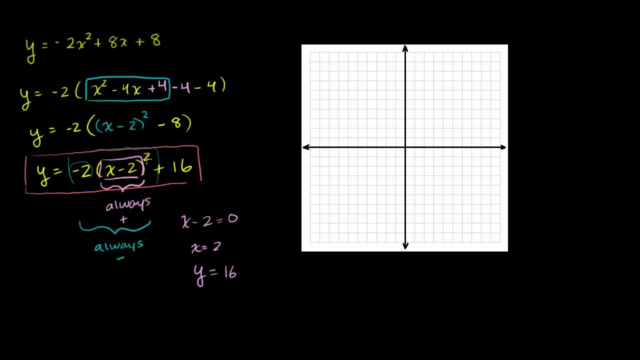 this quantity right here. it might be negative or positive, but when you square it it's going to be positive. When you multiply it by a negative 2, it's going to become negative and it's going to subtract from 16.. 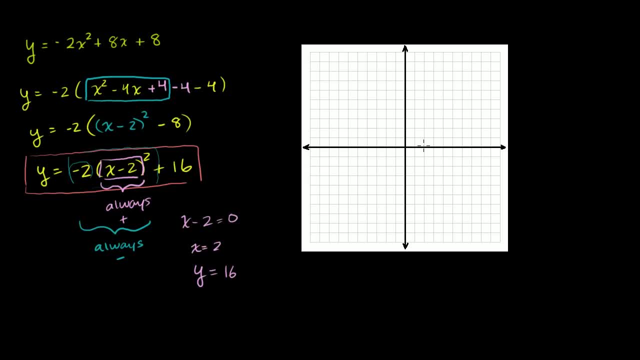 So our vertex right here is: x is equal to 2.. Actually, let's say each of these units are 2.. So this is 2.. And this is 2,, 4,, 6,, 8.. 10,, 12,, 14,, 16.. 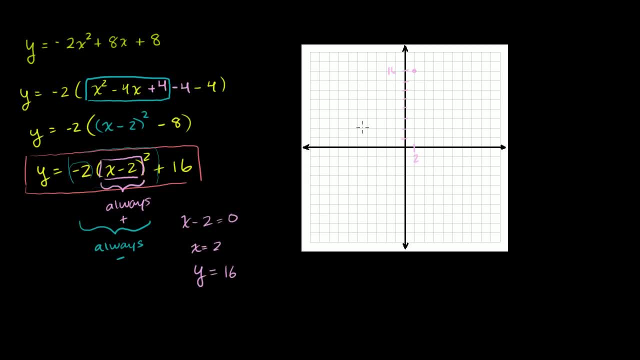 So my vertex is here. That is the absolute maximum point for this parabola, And its axis of symmetry is going to be: along the line x is equal to 2, along the vertical line, x is equal to 2.. That is going to be its axis of symmetry. 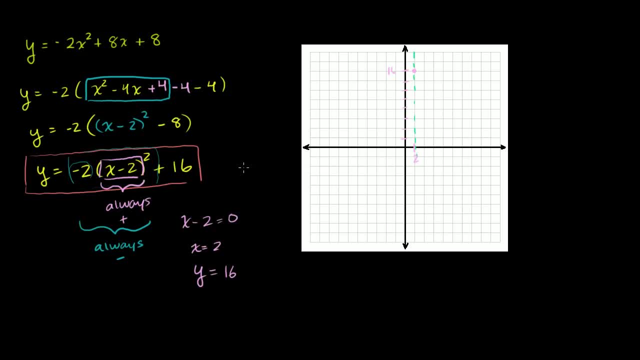 And now, if we're just curious for a couple of other points, just because we want to plot this thing, we could say: well, what happens when? I don't know? what happens when x is equal to 0?? That's an easy one. 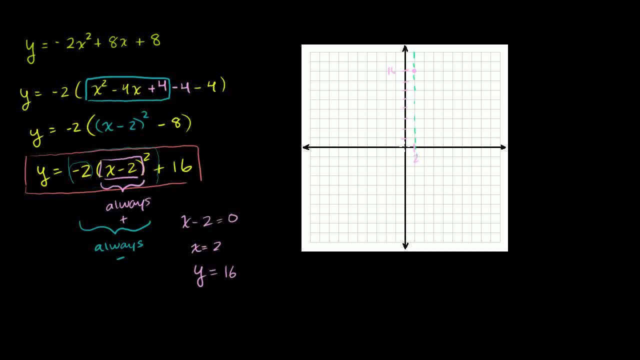 When x is equal to 0, y is equal to 8.. So, when x is equal to 0,, we have 1,, 2,, 3,, 4,. oh well, these are 2,, 2,, 4,, 6,, 8.. 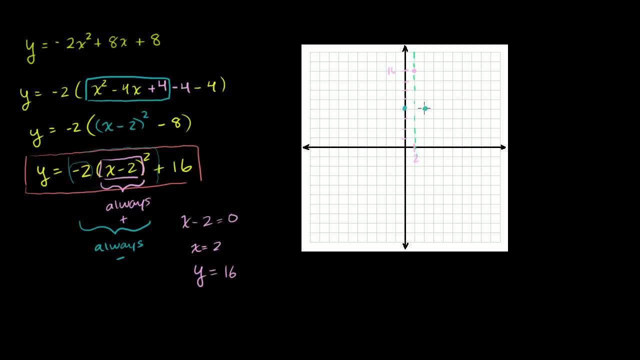 It's right there. This is an axis of symmetry. So when x is equal to 3, y is also going to be equal to 8.. So this parabola is going to be- it's a really steep and narrow one- that looks something like this: 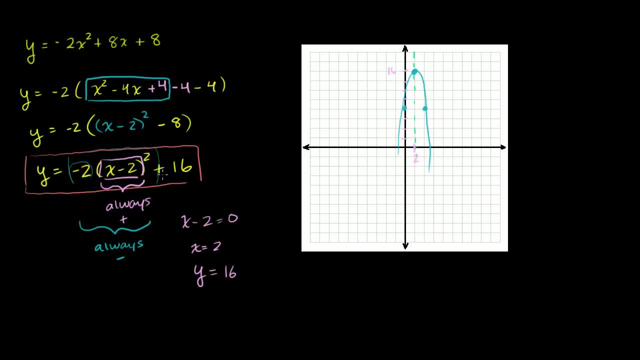 where this right here is the maximum point. Now I told you this is kind of the slow and intuitive way to do the problem. If you wanted the quick and dirty way to figure out a vertex, there is a formula You can derive it actually. 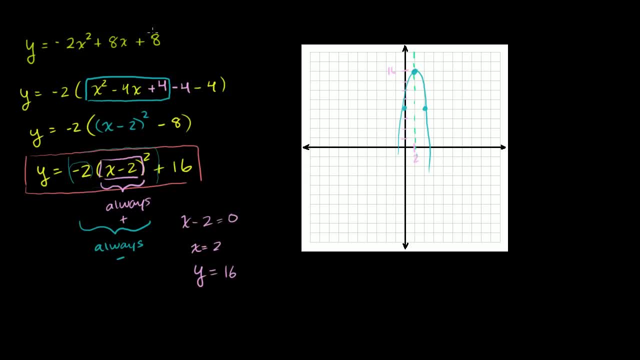 doing this exact same process we just did, But the formula for the vertex is x is or the x value of the vertex or the axis of symmetry is x is equal to negative b over 2a. So if we just apply this,